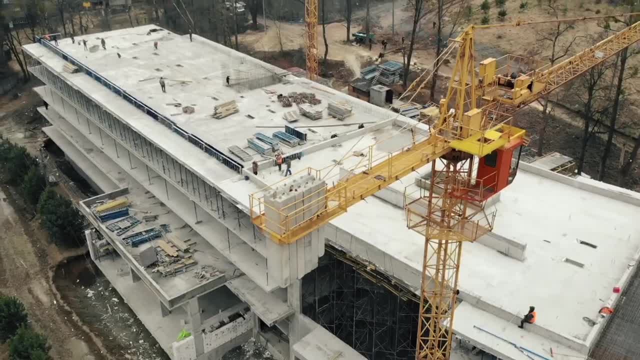 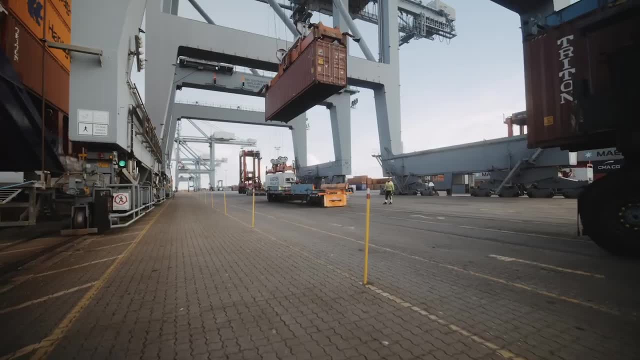 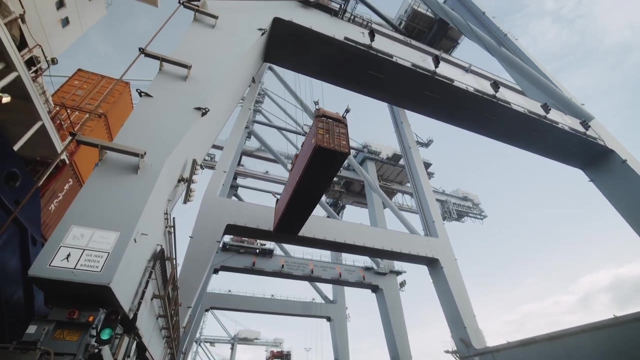 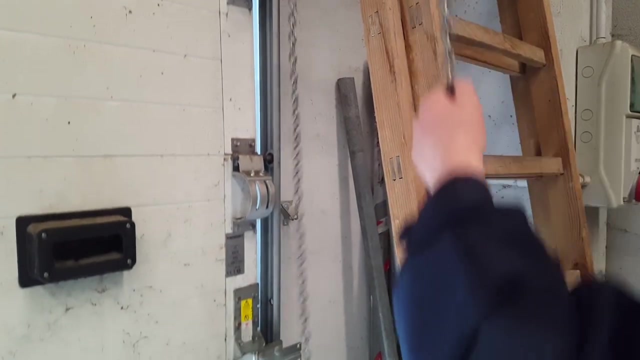 buildings or conquer bigger projects, it became increasingly necessary to be able to lift heavier objects. One of the main purposes of simple machines is to allow humans to lift much heavier objects than we can lift on our own. Two types of machines specialize in allowing humans to lift. 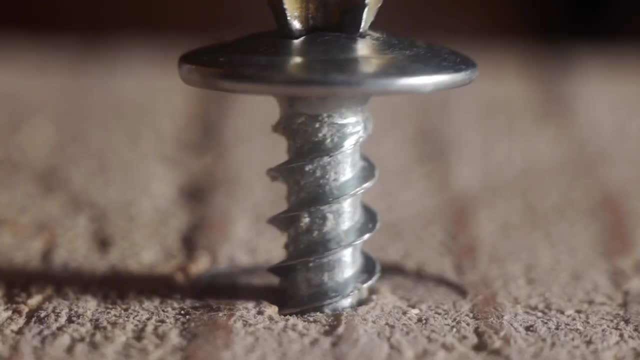 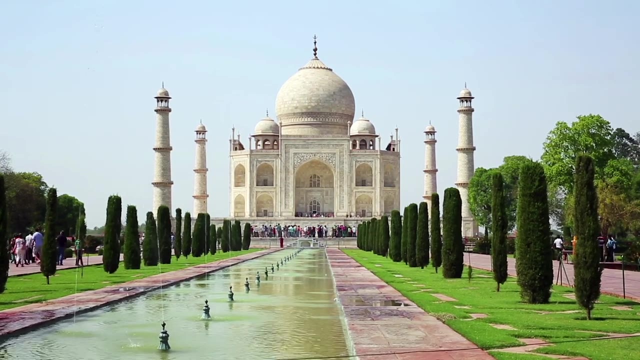 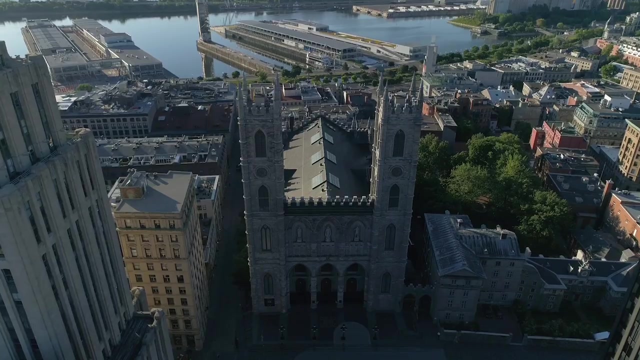 and secure extremely weighty objects, Screws And Pulleys. Without these inventions, humans would not have been able to construct buildings like the Taj Mahal in India, the Colosseum in Rome or Notre Dame in France. Let's first take a look at the humble screw. 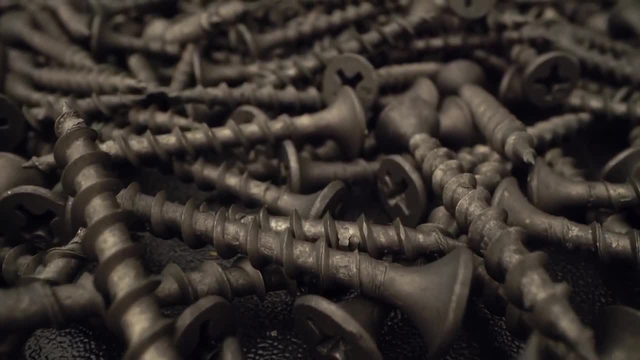 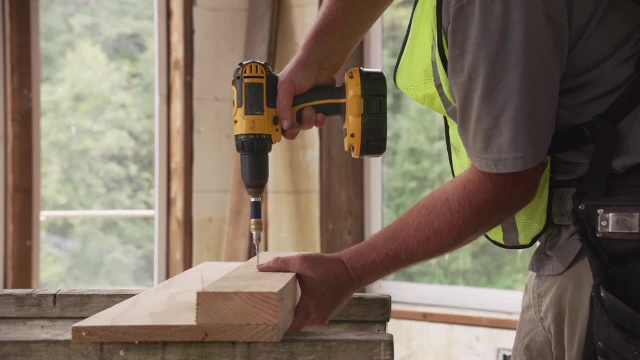 You are probably familiar with a screw that looks like this, but it is used to hold things together solidly and construct furniture, toys, electronic devices, homes and even a small house. It is used to hold things together solidly and construct furniture, toys, electronic devices, homes and even a small house. 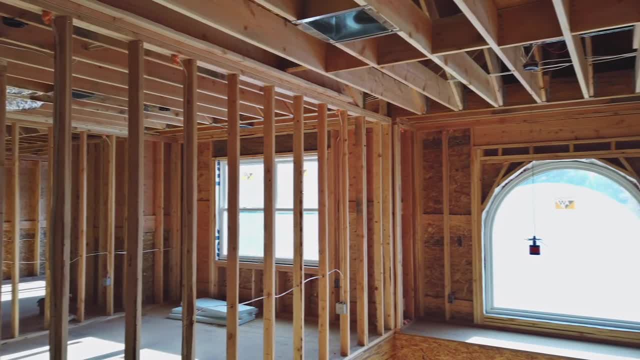 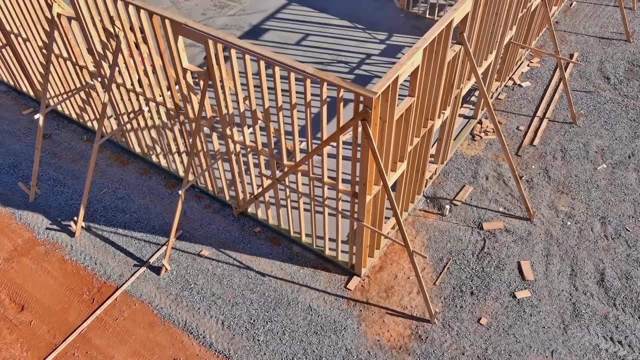 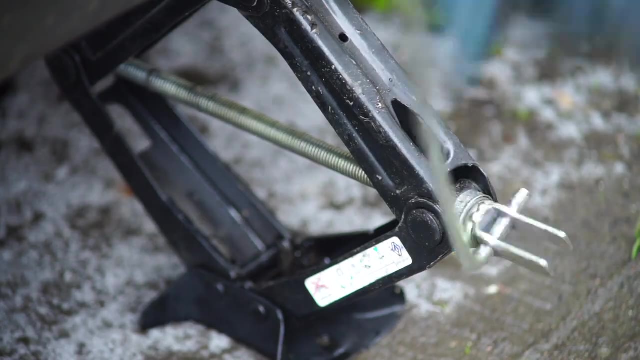 It is used to hold things together solidly and construct furniture, toys, electronics, screens, vehicles and buildings. You probably have thousands of screws in your home because they serve as an ideal way to secure and build the framing and walls. Do you now that screws can also be used to lift heavy objects? This is a screw jack. 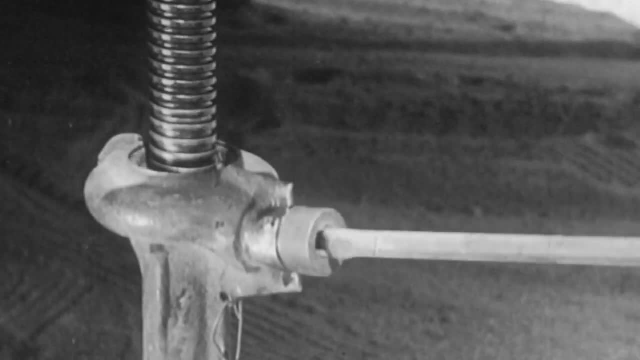 Do you see the large screw that it uses? A screw jack consists of a heavy-duty screw, a strong base to support beneficial, motivated objects in small hope. Sポ rəyную, this screw tip by the nature. karşıஙr Swoô pôn. 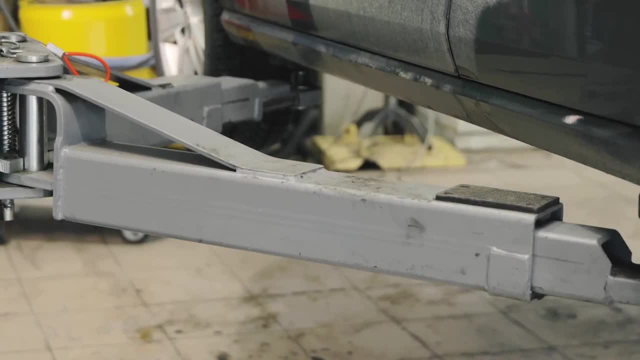 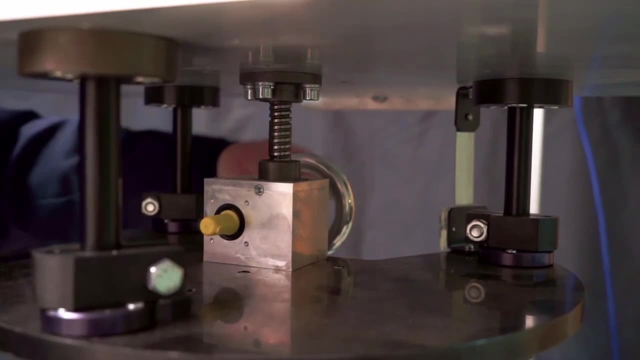 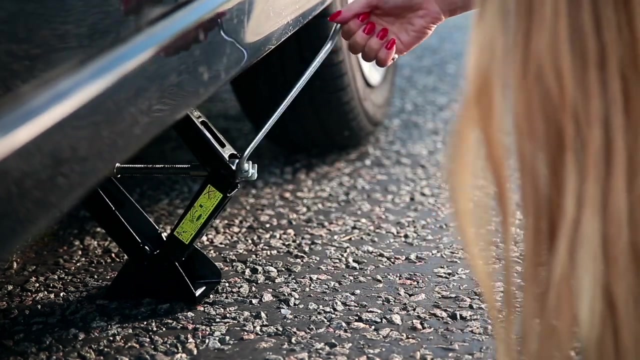 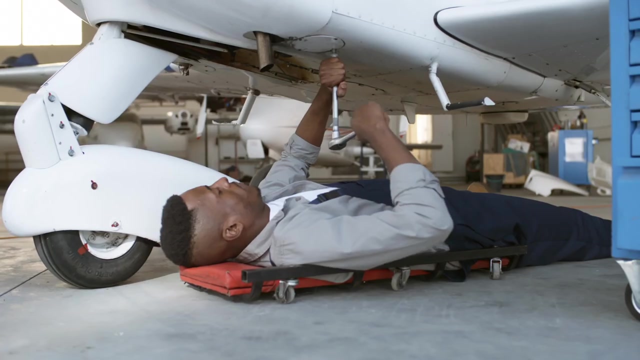 to keep it steady and a platform for holding a heavy object. Because the screw is actually a type of inclined plane, the screw will move higher and higher as it spins, raising the platform and slowly lifting the object. Screw jacks are most often used to lift cars so that they can be worked on, but they are 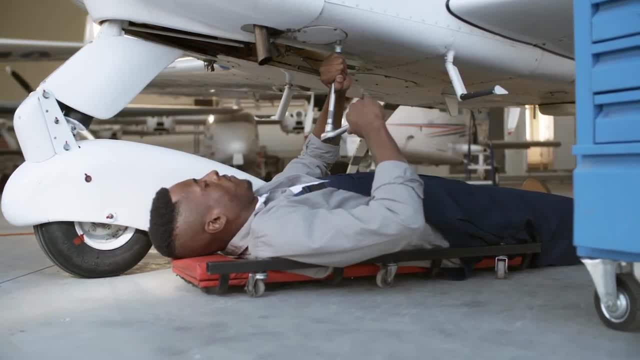 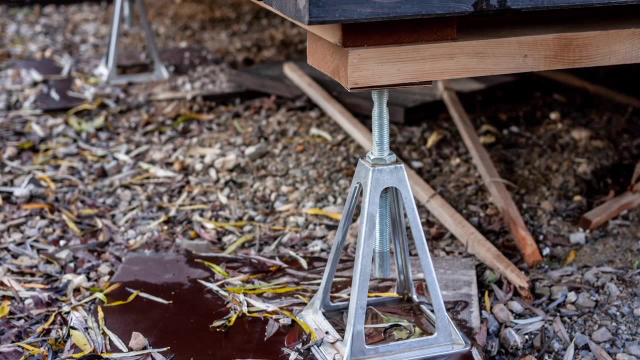 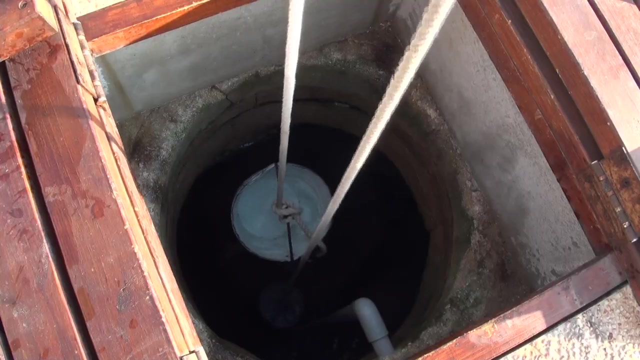 also used to move the flaps on the wing of an airplane, which is important for taking off, landing and controlling speed. Screw jacks have even been used to lift and level the foundation of homes or buildings. Another important, simple machine used for lifting is a pulley.